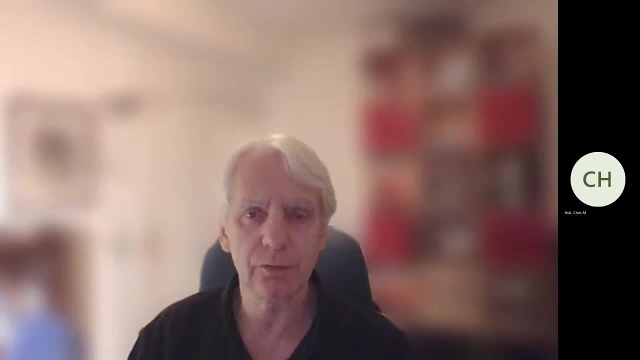 time with interactions governed by a small coupling constant And the theory was defined as a perturbation theory in this coupling constant. And that was a nice and very successful story. But then if one asks oneself what happens as the coupling constant becomes larger, 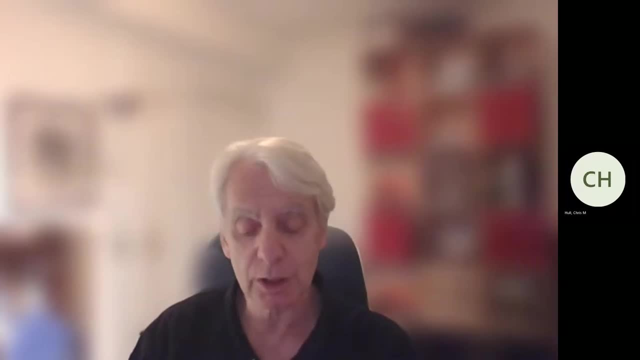 It's an interesting question which would start telling us about the non-perturbative structure of the theory. What happened in the mid-90s was it was realized that duality symmetries could provide the key to unlocking this non-perturbative structure. Roughly speaking, we can think about trying. 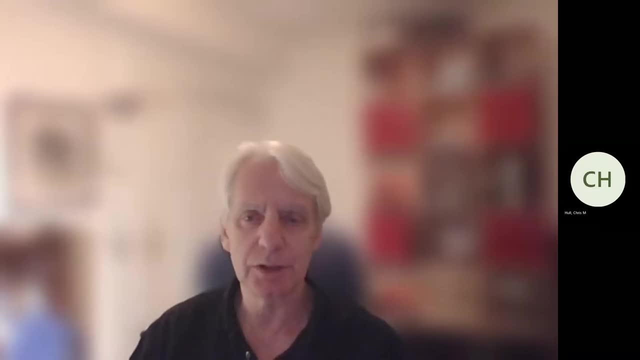 to understand the theory of large coupling as a perturbation theory in the inverse of that coupling constant, And that itself might be defined as a perturbation theory of a dual theory. But the theory of large coupling constant was one over the inverse of the one one. first, 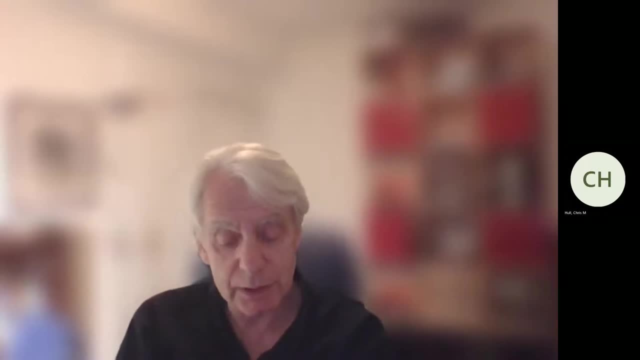 thought of, And this was the beginning of a set of ideas which led to big changes in string theory and into what has become known as the second string revolution, And I think it's fair to say that it's very, very much changed our view of what string theory is, so much so. 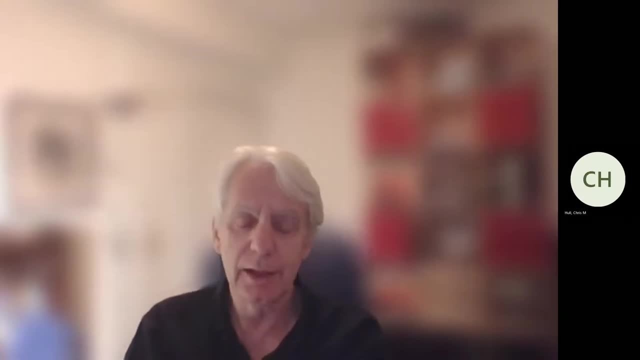 that it is no longer merely a theory of strings, And it's now To such an extent, then, that it was. the name has been changed so that now it's referred to as M-theory, And I'm particularly pleased to have a chance to talk about this body of ideas, as it's something 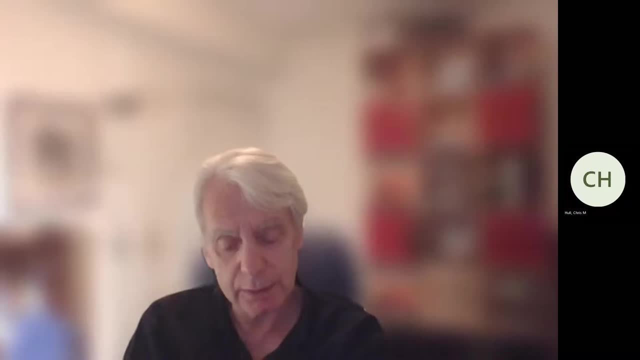 which I was heavily involved in my work in the 90s, and the two main papers which will be the basis of what I'm going to talk about are my paper with Paul Townsend from the 1994 and Edward Whitten's paper from 1995.. 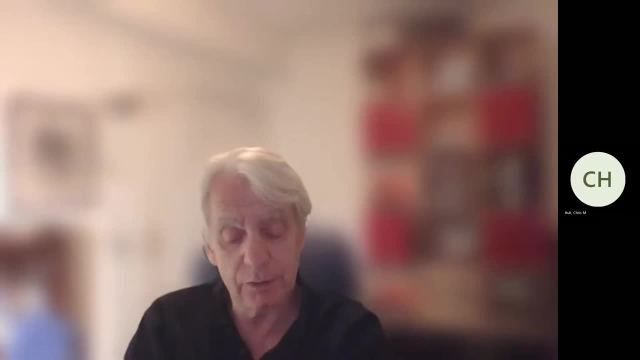 These laid the foundations, and then there's been a huge amount of work since then, And what I'm going to do is talk about some of the ideas from then, but with the benefit of the modern perspective and the modern understanding as to what's going on. 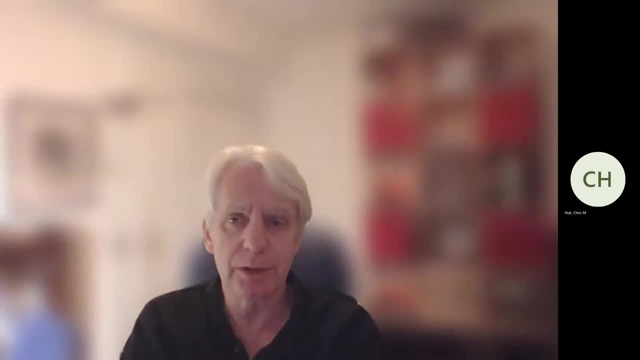 In preparing this lecture, I realised that there's a vast amount of material which goes into this, and to give full justice to it would require a whole lecture series. So what I'm going to do is I'm going to focus on some of the key ideas. 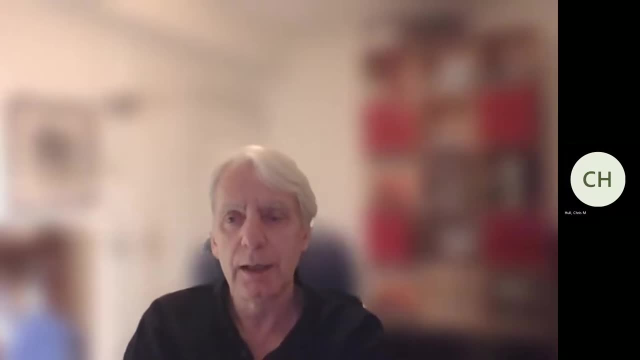 And provide references for those who want to read further, And some of the details and derivations will be the subject of some of the questions on the example sheet, which will lead you through some of the derivations and some of the arguments And we'll discuss. 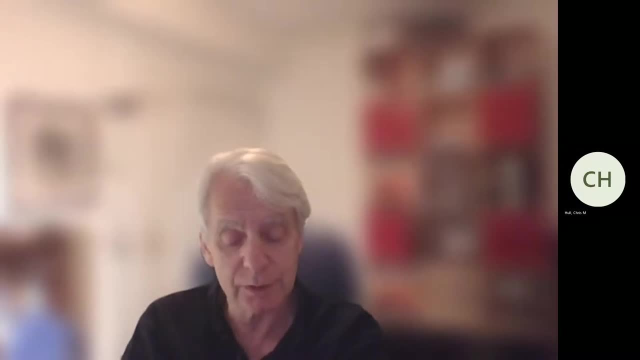 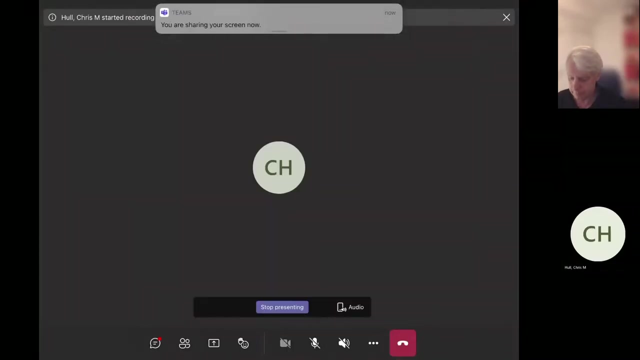 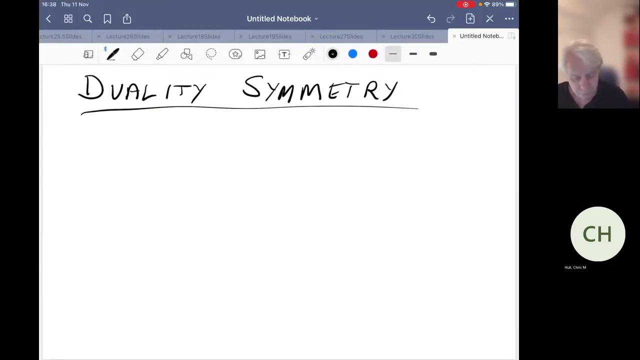 this in more detail in the follow up lecture where we discuss the problem sheet. So let me change now to sharing my screen, Thank you, And then I can start writing on my tablet. Good, So let me start by saying a bit more about what the story of what string theory. 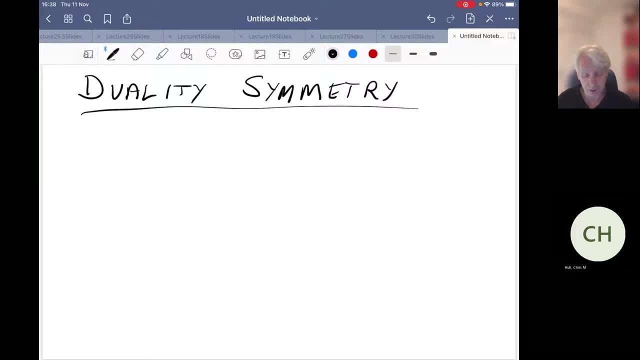 used to be was like, like, based on the perturbative structure. And let me start by thinking about, before going on to string theory, let me just make a few comments about the analogous statements for field theory. So the typical way of thinking about this is one starts off with a free theory. 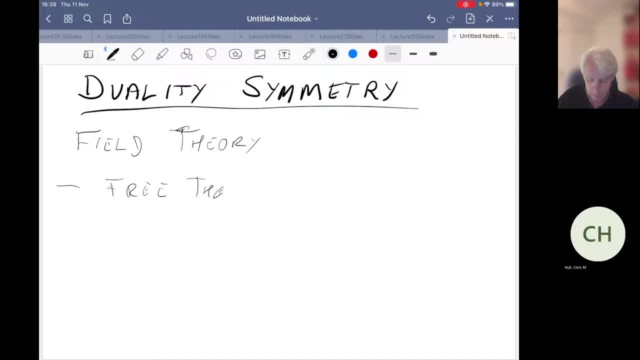 theory, a basic set of fields representing the fundamental degrees of freedom, And then one adds interactions, each of which is governed by a set of basic set of fields representing the fundamental degrees of freedom, And then the logical set of fields which is given by non-quadratic terms in the Lagrangian each. 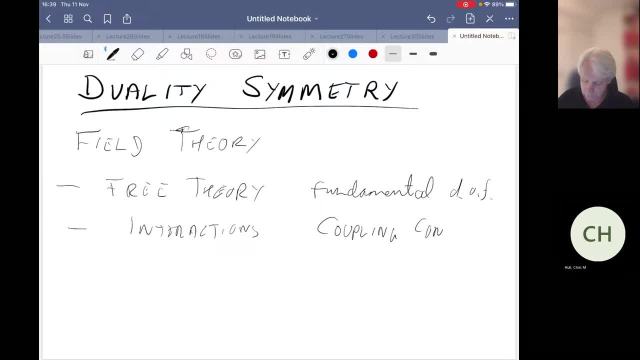 of which is governed by a coupling constant. So one has in general a set of coupling constants- lambda i- so that one might have interaction. here's a three-point interaction and there'd be a coupling constant which goes along with that And each interaction would have a separate. 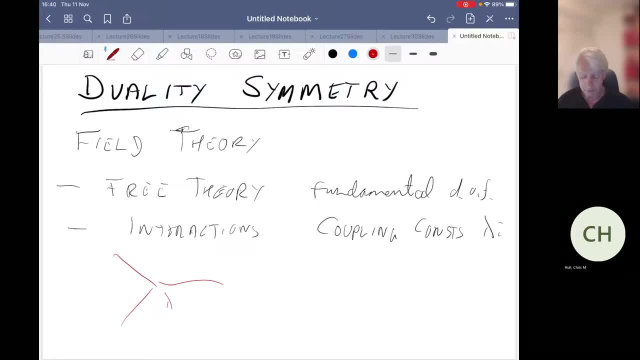 coupling constant, And then we could develop a set of fields which would be the standard theory in terms of um, a perturbation theory in these coupling constants, and there's a and but and there's a well-known um recipe for doing that, giving rise to a set of um. 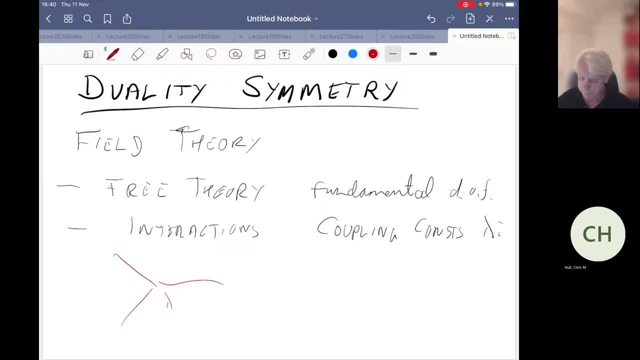 representation of interactions in terms of final diagrams, but um. so let's um think about, for example, yang mills, where one has um a field strength is the coupling constant time giving the um non-abelian terms. so here a takes values in the algebra of the, the algebra of the 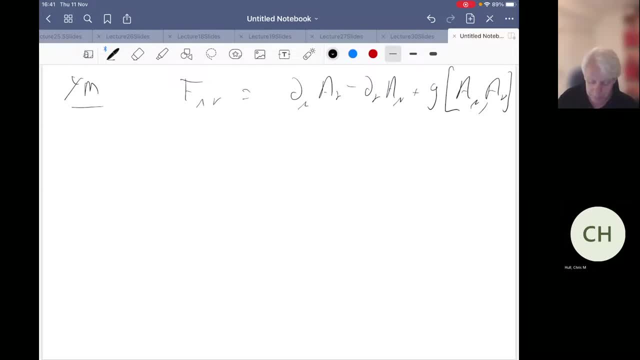 lee group. and then one has an action which is f squared, and um f mu nu, f mu nu squared, and uh, let's have a factor of a quarter, and here, uh, one could see that if one takes g to zero, one gets the free theory, and then um the adding the 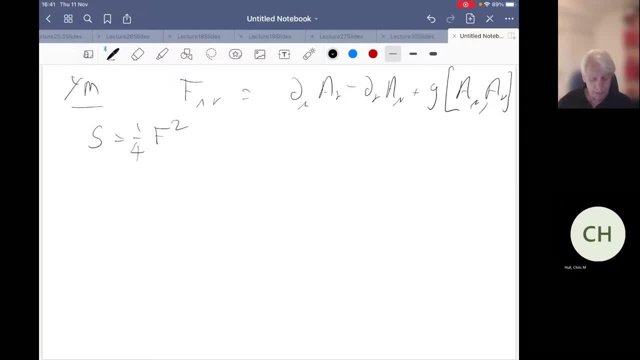 terms involving g, one's turning on the interactions and um. it's often useful to um, and so this gives the picture we were just talking about. but there's another viewpoint where, instead we take um, we rescale: define a primed equals g a, and then if one defines f, primed mu nu equals grad a, primed plus. 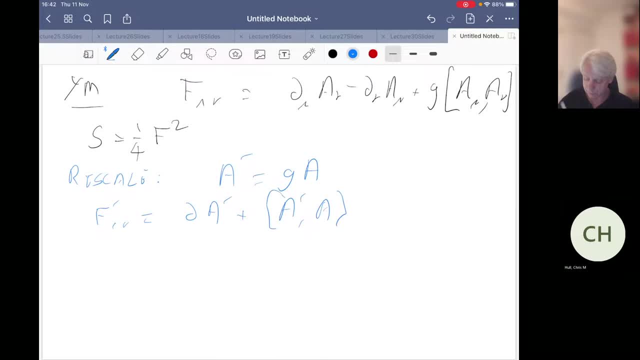 a primed commutator, a prime, the same index structure as before, but now um without the g. here this whole thing is just g times the original f mu nu. so now we've got a field strength where there's no coupling constant appearing in the interaction, and now the action can be written as: 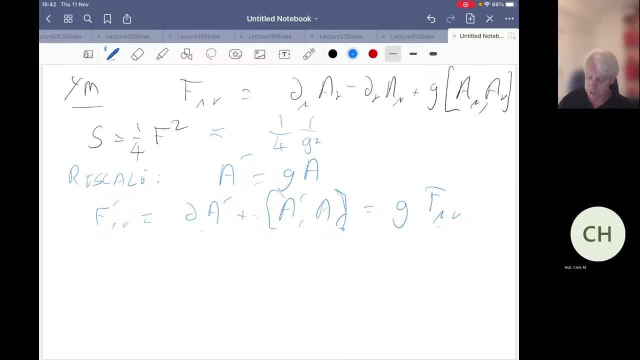 one over four, one over g squared. um integral of f prime square squared. So now we have the G primed outside the action as an overall factor and no term in the interactions, And then in the functional integral we have, you can write it as DA. 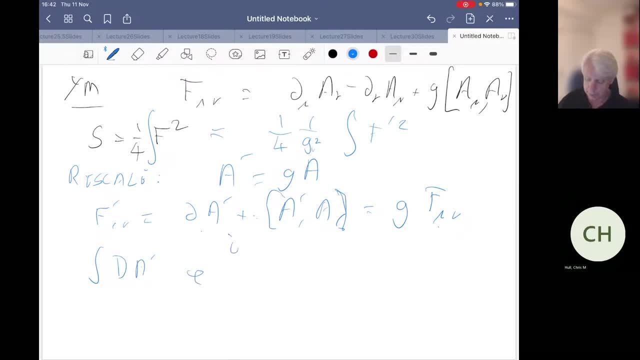 primed E to the I 1 over G squared, and there's the usual H bar, then integral of F, prime squared, And here we see that H bar G squared always appear together. There's no other place. the G has been rescaled out of the interactions And so the coupling constant. 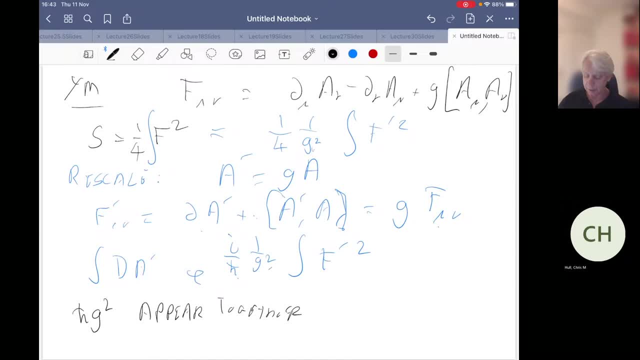 just appears outside the action, the same place as the H bar does in the functional integral, And so can We can absorb. We can absorb H bar into G squared. And this is, this combination, is the loop counting parameter, so that at L loops one has a factor of. 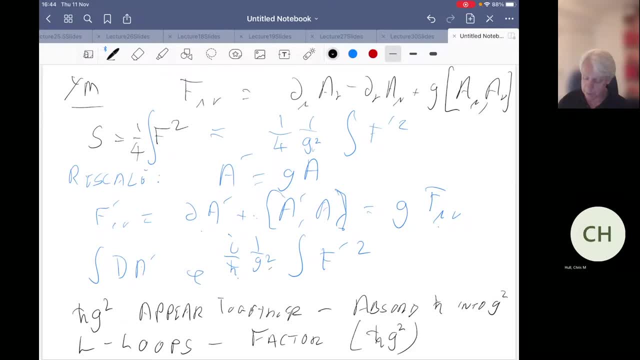 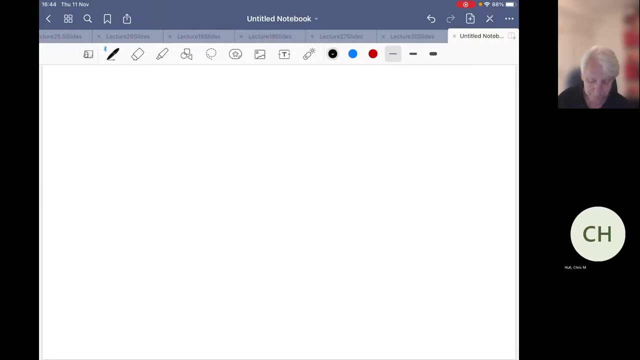 H bar G squared. This, This is L number of loops minus one. so at zero loops or tree level, we have the one over g squared that appears in the action and uh of an l loop contribution will be of order l minus a factor of l minus one, so that, um, if we were to look at an interactions, we, um, we might have a tree level. 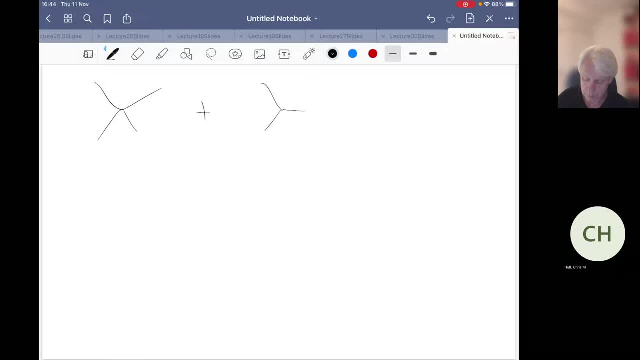 interaction plus a one loop interaction plus a two loop interaction. so we'd get a factor of one over g squared overall. we get one plus g squared plus g to the fourth, and so on. appearing here, appearing here, um and um. so that gives the standard picture for um. 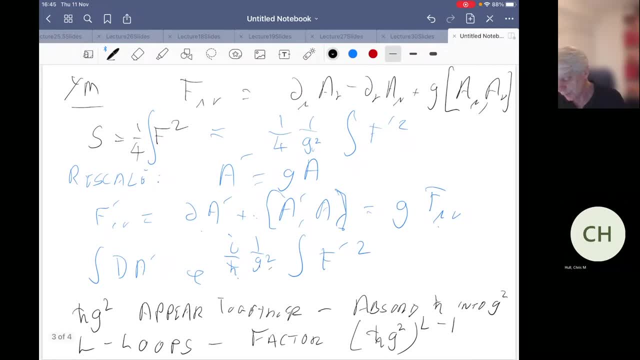 perturbation theory. i've just talked about the example of yang mills. um this, one can look at similar rescalings for the other fields and um one can, one could always one can- rescale so that the um coupling constant is outside. and the reason i'm going through this rather elementary point. 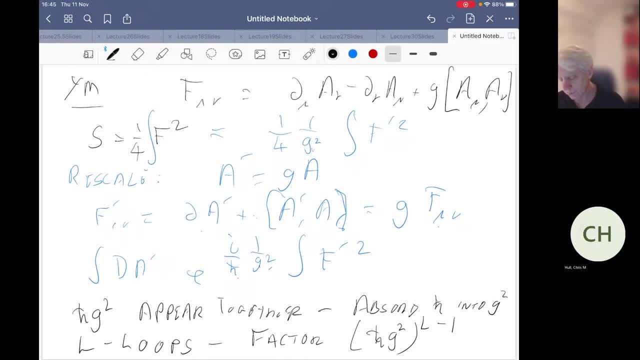 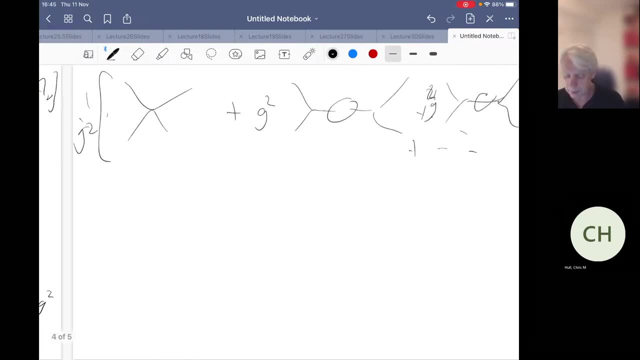 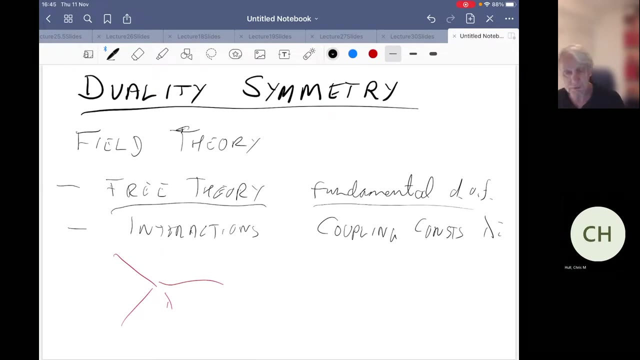 is that there's going to be um, a rather similar point which comes in string theory, in that there's two different ways of thinking about the interactions. so let's talk about um. but a key ingredient here, of course, was starting off with a free theory, and it required us to know what the fundamental degrees of freedom. 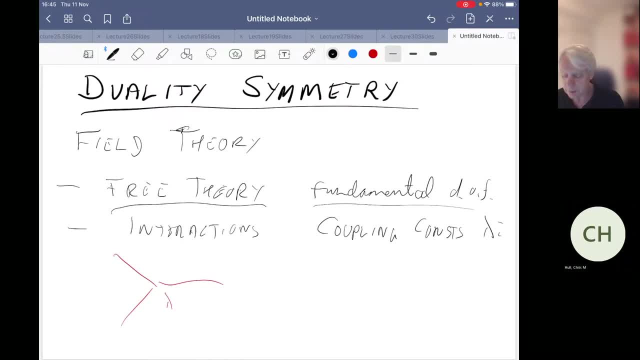 are, and then we'd think of the theory as set, uh, setting up some interactions for those fields. so now let's turn to theory. let's just describe it: string theory. so the basic picture is that we might have, for a closed string would be a loop of string um, which would move through space time. and as it moved through space time, 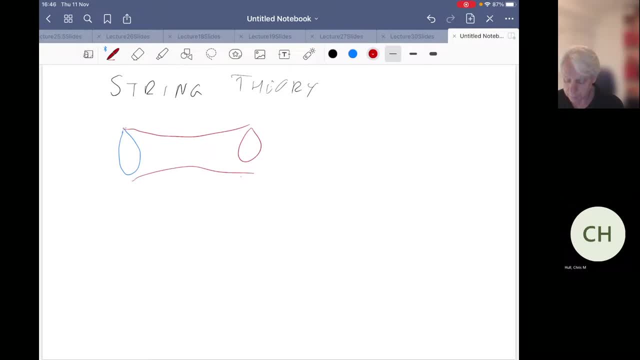 it would sweep out a cylinder. so here i'm thinking about time as moving in this direction. and um, there's. the action for this is then given by the function t. okay, so t times the area swept out by the string. so this two-dimensional surface will have: 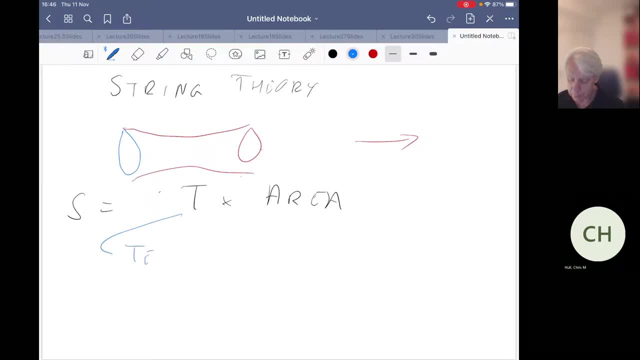 an area and that's the action, and this t is the tension, and it's some type t which is sometimes written: it's got the dimensions of one over a length squared, So it's sometimes written as one over a particular length scale which is defined in this theory, which is the length, the string length. 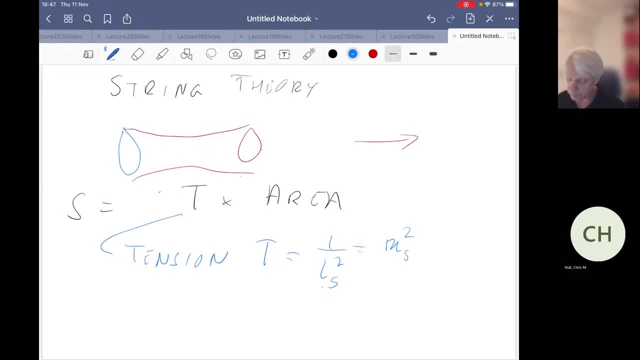 You could also think of it as defining a mass squared, a string mass, And historically it's given by a parameter known as alpha prime. So this is one over two pi alpha prime And there's a fundamental length scale which is introduced to the theory, or a fundamental tension. 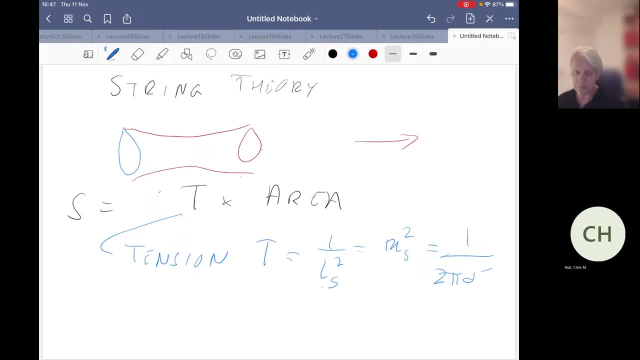 A fundamental dimensional quantity And this sets the standard length scale of the string and typically determines the typical size of a string. And in the theories we'll be talking, in the fundamental string theories, this string length is of the order of the Planck length, the 10 to the minus 33 centimeters. 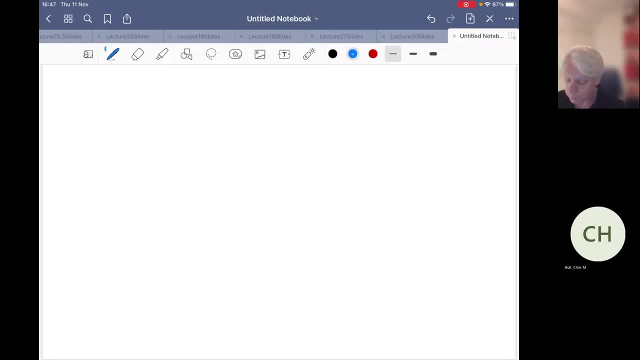 This gives rise to. if one looks at the string length, it's of the order of the Planck length, And if one looks at the quantization of this, this gives rise to the excitations of the string give rise to an infinite set of particles. 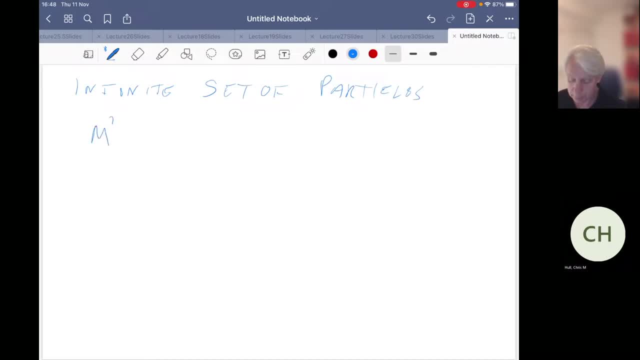 With masses, m squared in units of the string, mass squared minus one, naught one, two and so on. So first of all there's a mass, something with mass squared negative, which is a tachyon, which is bad. 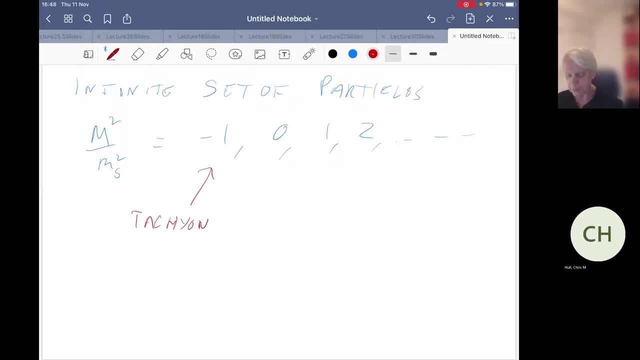 It's a signal that this particular theory has got a field with negative mass squared, which is usually interpreted as meaning that there's an instability in the vacuum, And so that would lead to formal problems with the theory. But mass zero: we have some massless fields which include a graviton, an anti-symmetric tensor gauge field and a dilaton. 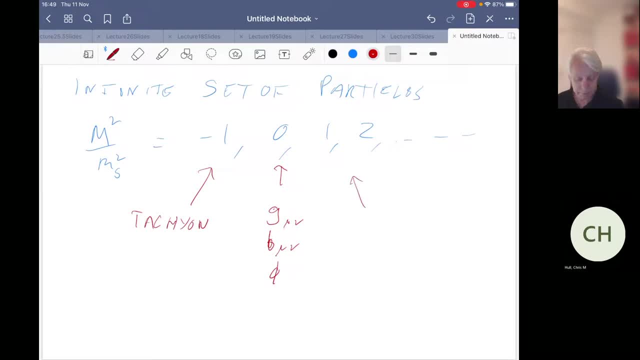 And here we have an infinite tower of massive fields which typically, as we increase in mass squared, they typically give rise to fields, some higher spin fields with lots of indices, But mass zero is now a spin field that is constructed by some kind of partial SPало, matching together with lower spin fields and higher things. 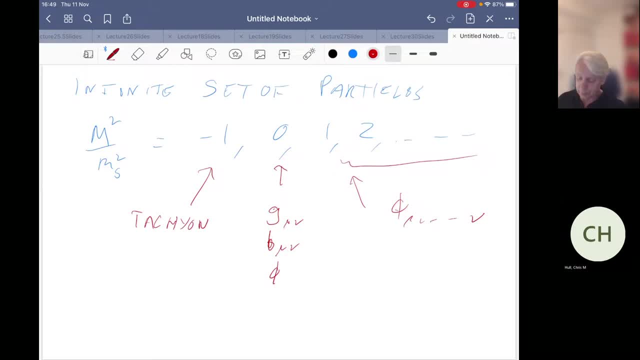 And we can think of it as a two-dimensional field theory. If we, if on the string world sheet we introduce a coordinate, and of course we can think of it as a battery, It wouldn't be a problem if it wasn't aziehable, but rather a very steady string. And so the distribution of the probability would be the same. here Theンタiline of the rating and the machine can be really interesting. So it's always good to get the probability right. The entire function is always good, The entire function of a part of what you have. 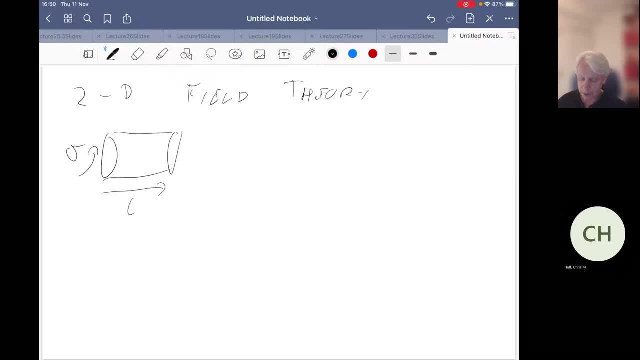 And so the distribution of a part of what you have is always good And we look for the probability. But actually I think we're just trying to work with you, So we kind of have to get the probability right: sigma around the circle and a tau describing the proper time of the evolution of the 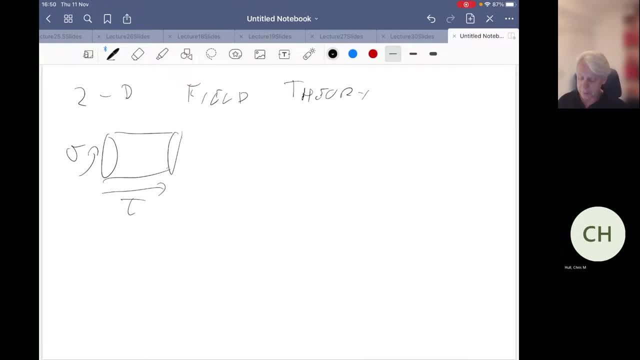 string, then the embedding of this cylinder in space-time is given by space-time coordinates dependent on sigma and tau, and then we can think of these as two-dimensional fields and the action as giving a two-dimensional defining, a two-dimensional field theory which is designed so as to extremize the area of the um of the world sheets embedded in space-time. 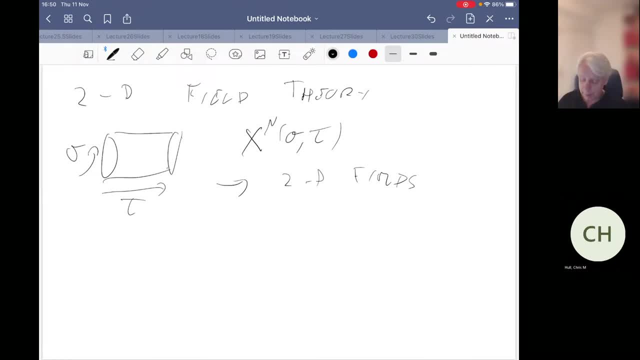 we can, uh, we can all we can. this is the basic bosonic string theory. we can um modify this by adding 2d fermi fields into a set of fermi sonst fields, and um it could be done this: it turns out that this could be done in in a consistent way. 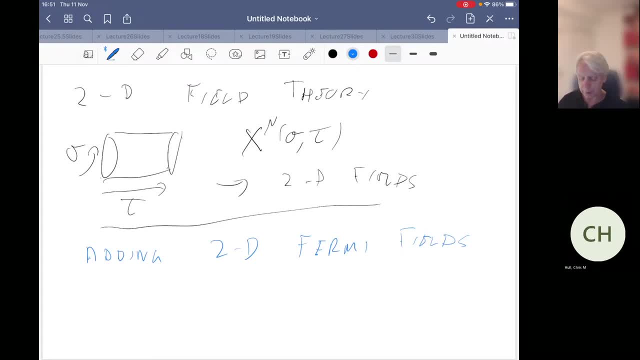 um. so, first of all, introducing these thermy fields could be thought of as, roughly speaking, introducing um, fermi on currents moving around the loops of the string, and um in defining the. looking at the quantum theory defined by the bosonic string or the fermion, It turns out there are very stringent restrictions required from requiring the consistency of the theory. 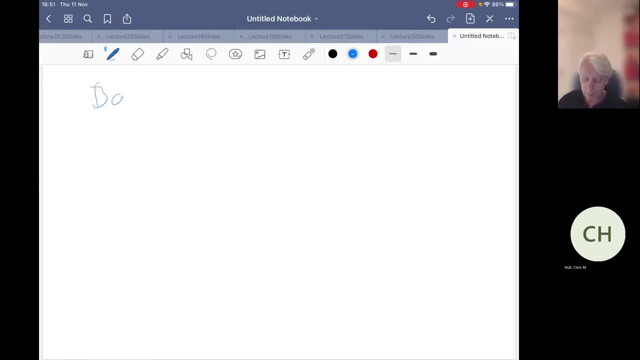 For the bosonic theory it requires the spacetime dimension to be equal to 26. And for the ones with fermions it turns out that the dimension it only works for spacetime dimension 10. And then the theories which emerge have spacetime supersymmetry, rather remarkably. 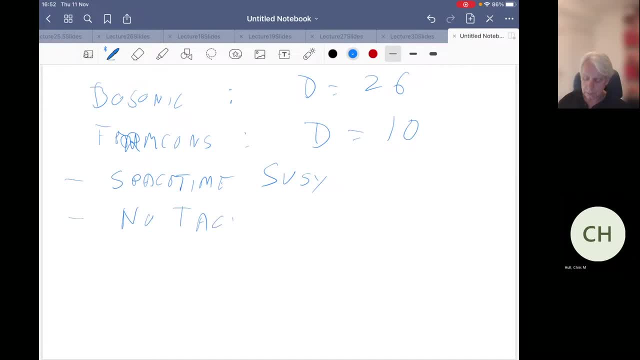 They have no, No tachyon. so there's no negative mass squared term, so there's none of the instability. So if we look at the spectrum of strings, this term is missing And we'd start off with massless fields. 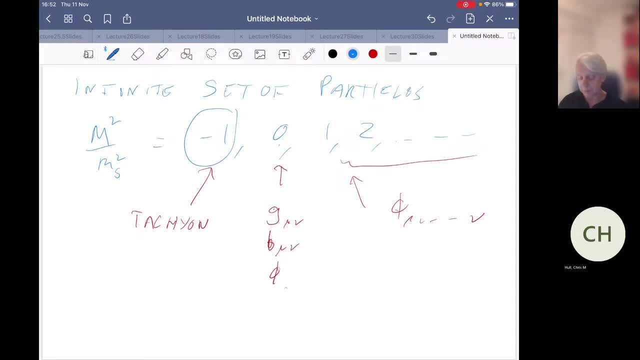 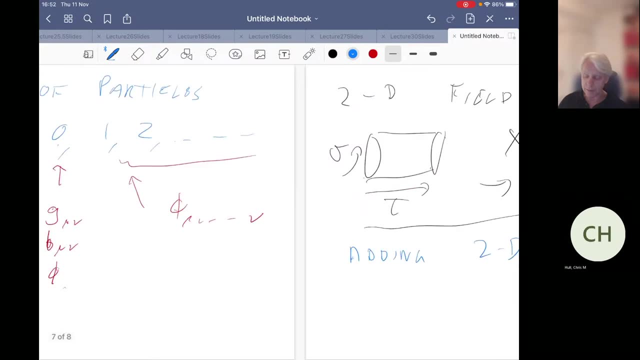 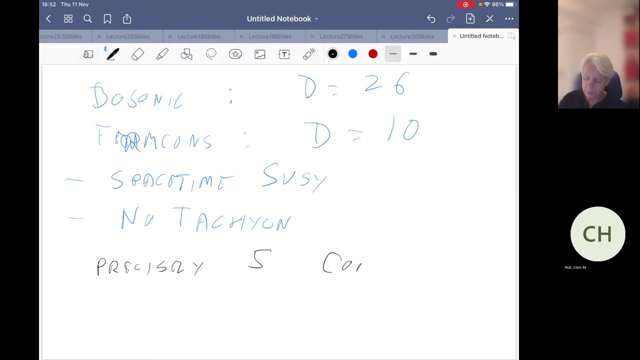 Which include these plus their spacetime superpartners, because it's a supersymmetric theory Plus super multiplets of all of the mass of higher massive strings, higher massive string modes And, Rather remarkably, there are precisely five consistent theories which arise in this way. 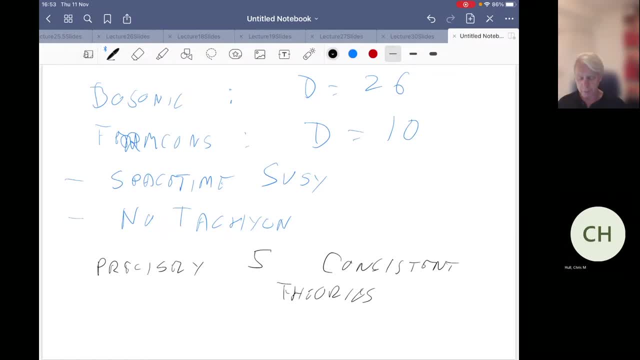 Each of which looks different. They've got different kinds of fermions introduced into them, But nonetheless each of them appears to define a consistent quantum theory Which gives ultraviolet finite amplitudes And in particular, it has. These are quantum theories which include gravity. 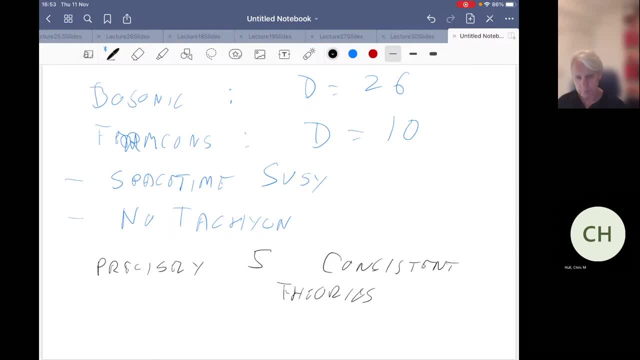 So it gives Each of these gives a candidate for a consistent quantum theory of gravity. Now, one of the problems here is that. So one of the issues which immediately arises is: why are there precisely five Consistent quantum theories of gravity arising in this way? 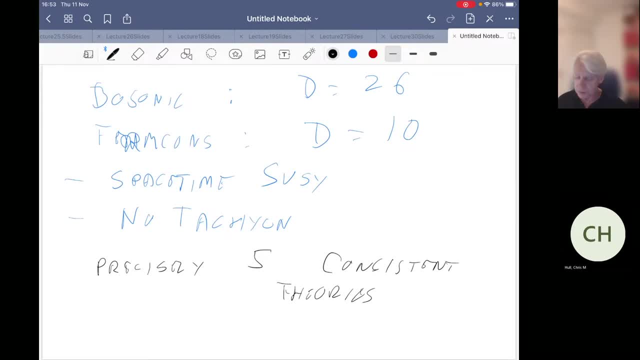 And That's one of the questions I want to address in this lecture. So another feature is that the massless sector, as I've mentioned, Is a supersymmetric Theory which includes a set of particles, including gravity, So it's A supergravity theory. 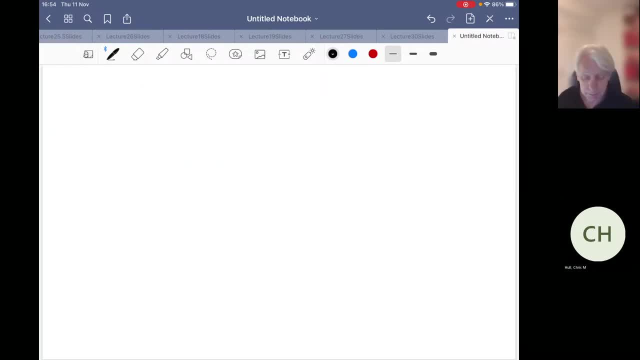 So what about introducing the interactions? So One can think of it as, Analogously to the way we talked about interactions With field theory, We can think of Having a smooth surface which describes One string. We think of time moving left to right. 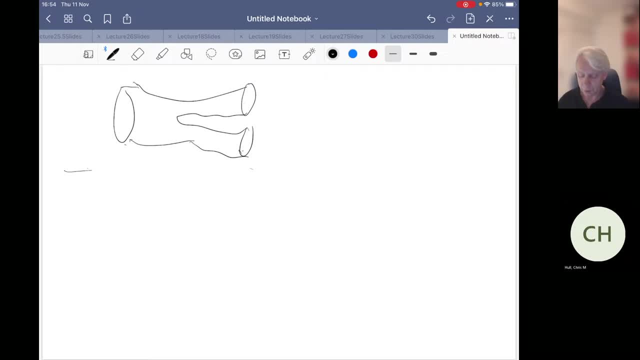 It's, You have one string breaking up into two strings Or, reading backwards, two strings merging to form one string, And we can introduce the coupling constant G associated with that. We can also think about the analogous statement structure. So in this case, 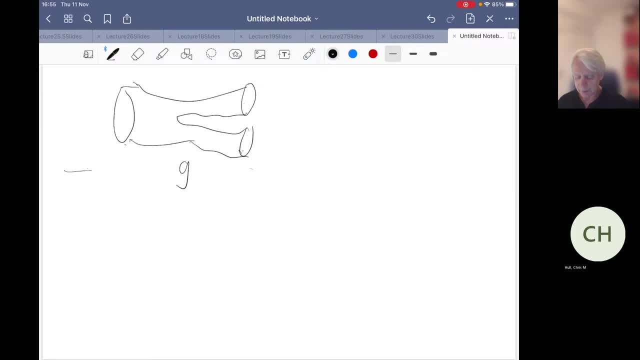 We think of the free string theory Together with Small, With perturbative interactions, And We can also think of rescaling things so that The, The G, Instead Counts the number of loops. So this way of looking at things is the thing which arises from some approaches to string theory, such as: 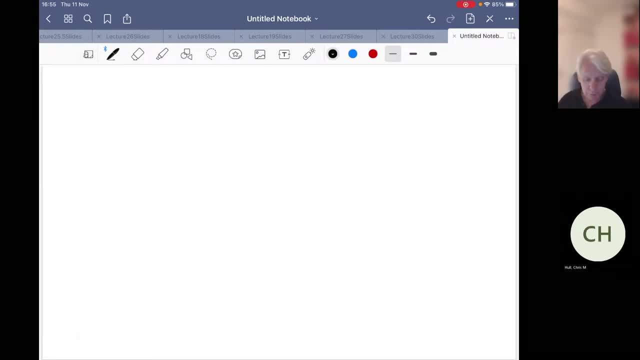 String field theory And the world sheet approach, which I want to talk about. We can, We go to What stone is the String frame? And we have a natural picture of The, The string interactions in terms of Expansion, in terms of the number of. 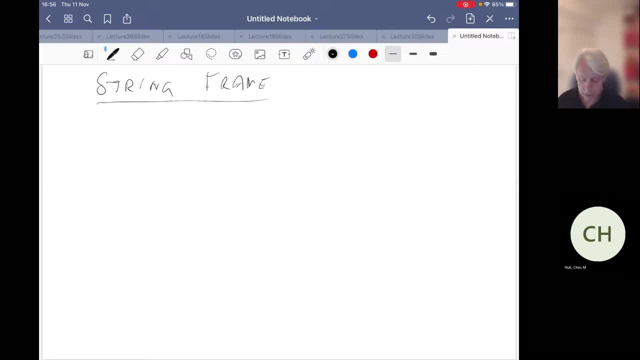 In terms of strings moving through space time, So the world sheet approach, So we can think of it as. So, if we're looking at a four point interaction, We can think Of the interaction between four string states, Four asymptotic string states, 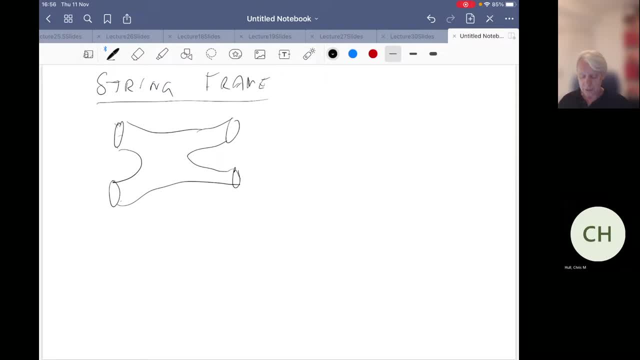 As Thinking about it as having a world sheet Which joins all of these up together. So the way I've drawn it, we're thinking about two string states in the far past Coming together, Merging to form one large closed string. 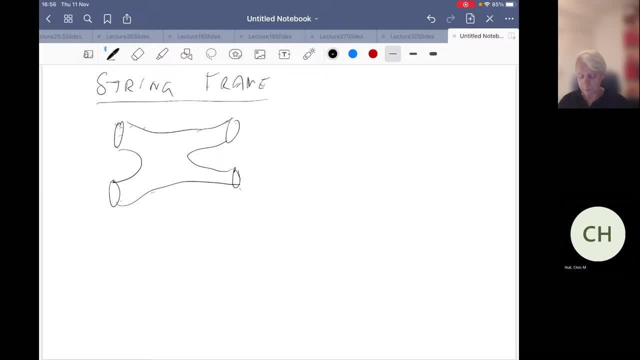 And then It's breaking up to form two more, So that we're getting a process which got Two states in going to two states out, And the The picture is that one would choose the asymptotic states And then one would sum over all possible. 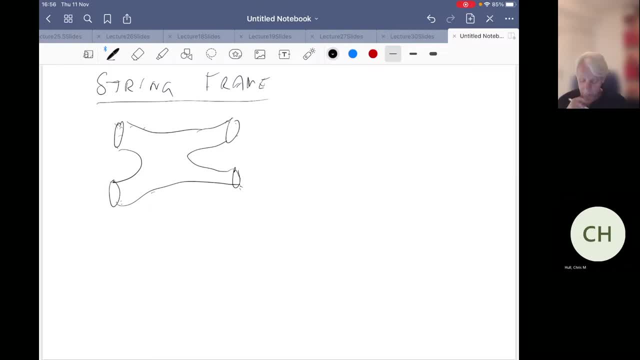 Surfaces which interpolated between those And there would be a loop expansion for this. We could think of this as This plus A bay area Which has two holes, So that's going to be an interaction of, Of two different kinds of. 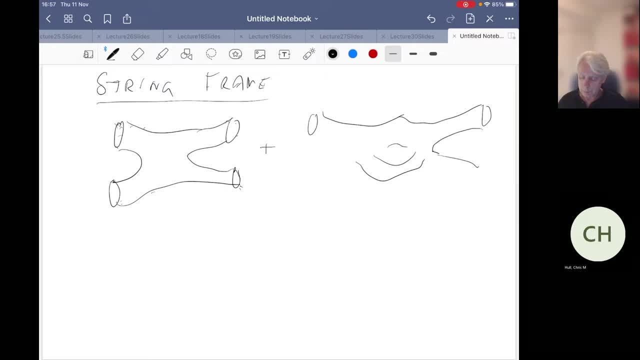 Two different kinds of Uniforms. Actually, We could have this as one One wave, But it's more like All three of them. So that's going to be the One wave And from One of them. How about this? 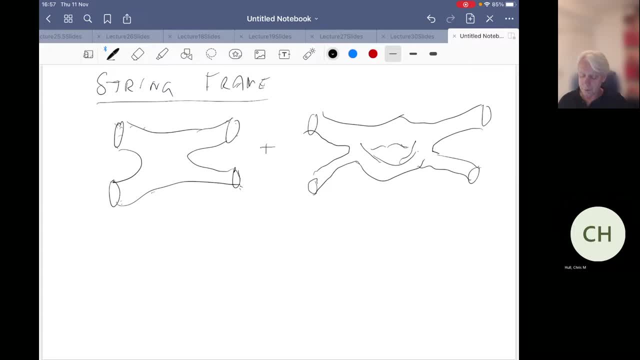 We can think of this as The圧ol, As Subtracted From All three of them, And then we could think of this as: How about this Subtracted? So this would be The, The, The. 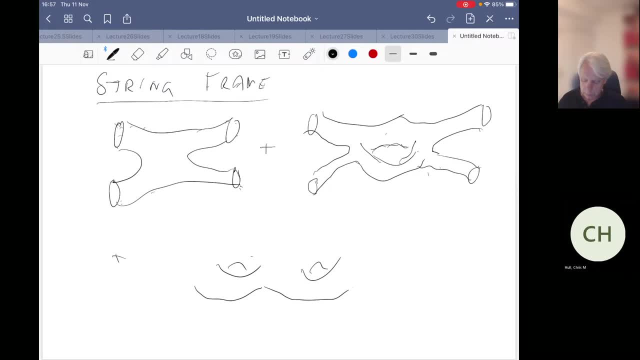 Subtracted. It had two holes in it. So here we can think of this as two doughnuts glued together and then four cylinders glued onto that and so on, And we can think of this as being So. this would have a factor of one over G squared. 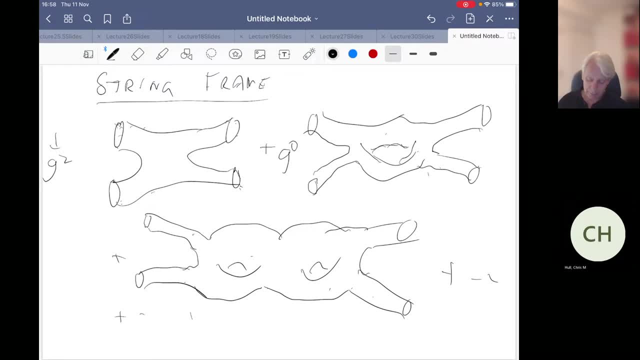 This would have a factor of G to the zero, This would have a factor of plus G squared And in general we'd have G squared To the genus, minus one, where the genus of the surface is telling you about the number of holes. 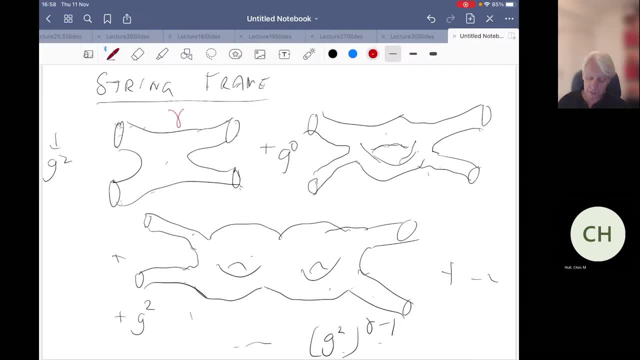 So this is genus zero, this is genus one, this is genus two, and this is telling us about the genus of the basic underlying surface on which these tubes are glued onto. So this is saying that we're gluing four cylinders onto a Riemann surface of genus G. 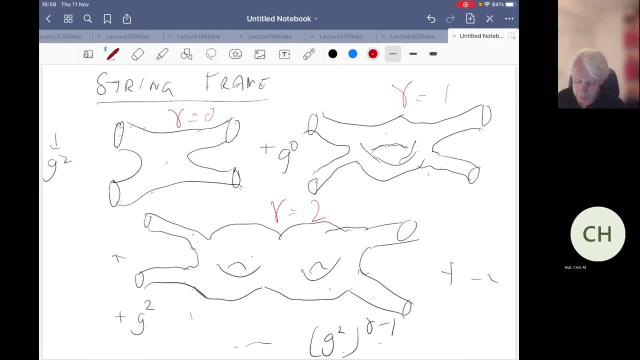 So in this picture we sum over all surfaces, we get an expansion in G depending on the genus of the surfaces and as a result, we get a picture for the perturbation theory, for the expansion, for the scattering amplitudes of string theory. 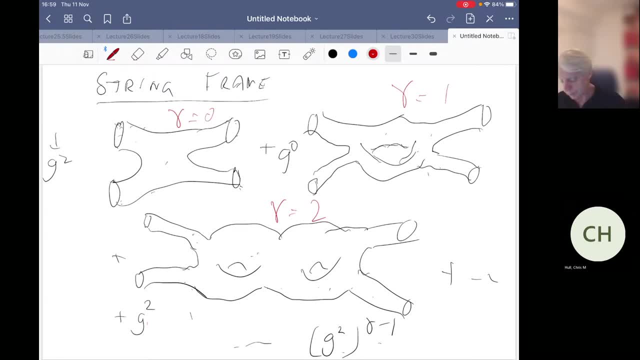 And in each case we get a factor of G squared, We get a power series. It's in G squared And if G is small we can think it gives a good perturbation theory. One of the features of superstring theory is that in each genus the amplitudes will. 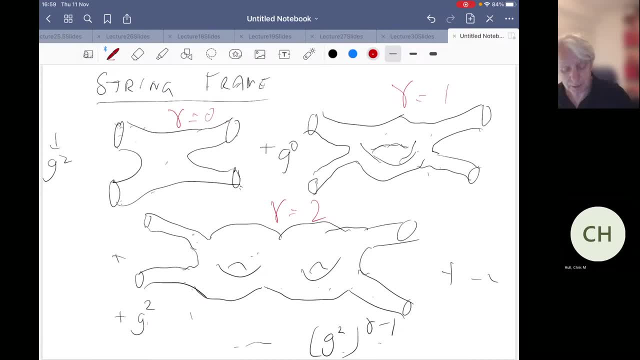 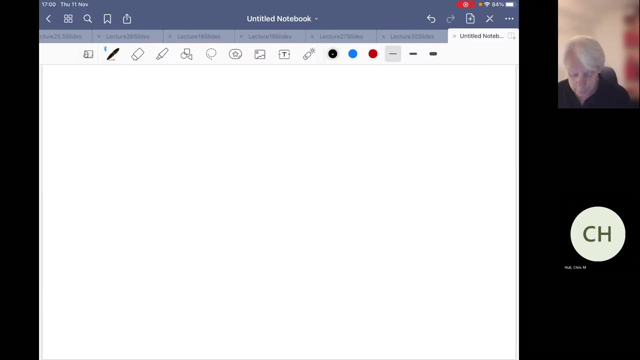 each be separately well-defined and have good ultraviolet properties. In the world sheet action We have the integral over G, sigma, G, tau. we introduce a metric on the world sheet and let's have indices- alpha and beta- running over two variables, where alpha equals zero. 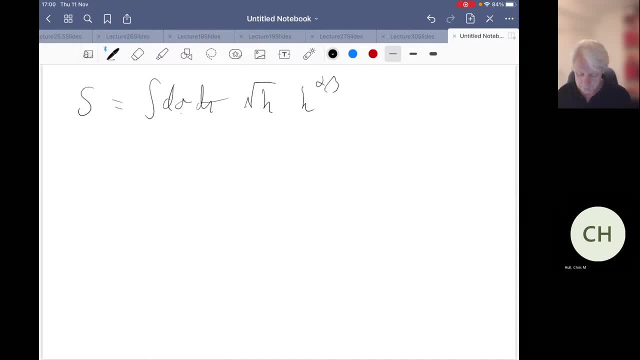 corresponds to tau and alpha equals one corresponds to sigma. So we get grad alpha X mu, grad beta X mu, And then we have the integral over G, sigma, G, tau. we introduce a metric on the world sheet and we have indices- alpha and beta- running over two variables, where alpha equals zero. 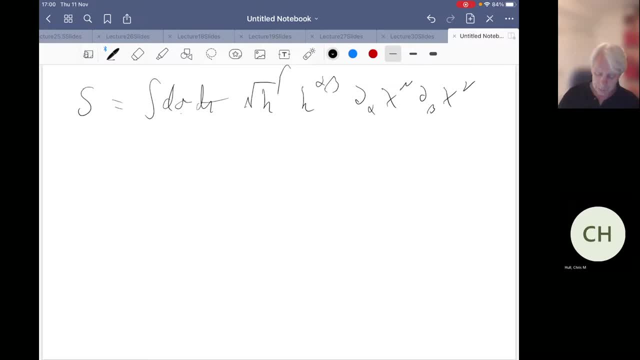 corresponds to pull off, And then again, at level 3, we get X mu, which is the basic action rule. So with this, just this action on its own, extremizing this will give rise to extremizing the areas worked out by the world sheet. 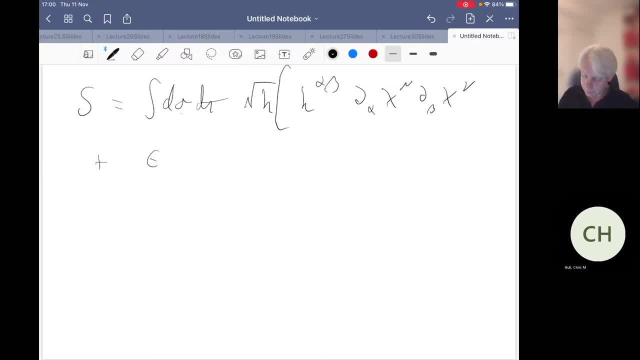 And then there's the coupling to the space-time metric G, mu, mu of X, And if the space-time metric is not constant, then this describes a nonlinear action, which nonlinear dependence on x, and so this is described as this called a nonlinear sigma model, and then 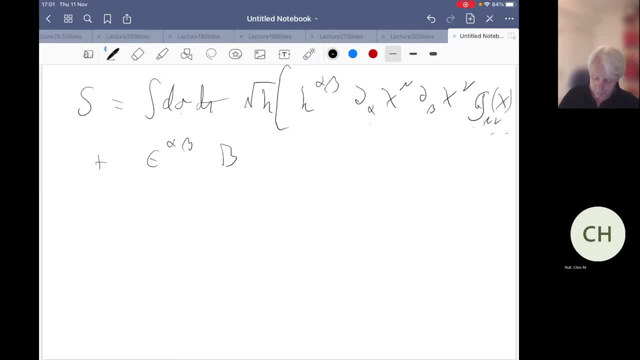 there could be a coupling to a b field, which we introduced by using an epsilon tensor on the world sheet, b, mu, nu, grad, alpha x, mu, grad, beta, x, nu. and then there could be a coupling to the scalar field. so this is the so, looking at the couplings to the massless fields in the action, we've got a massless 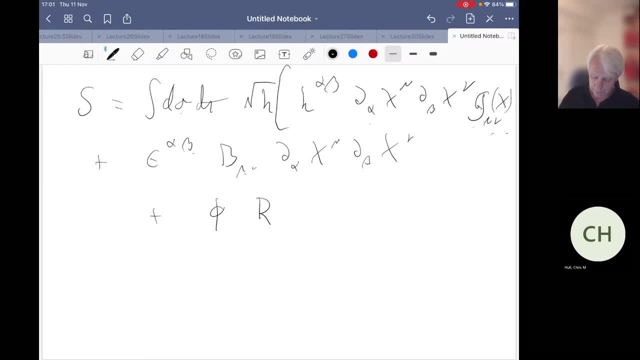 graviton, a massless b field, and this couples to the scalar curvature of the world sheet metric h. and let's put in a factor one over four pi. now it turns out that integral of one over four pi times r, h, r, d, d, sigma d tau equals, is precisely equal to um. 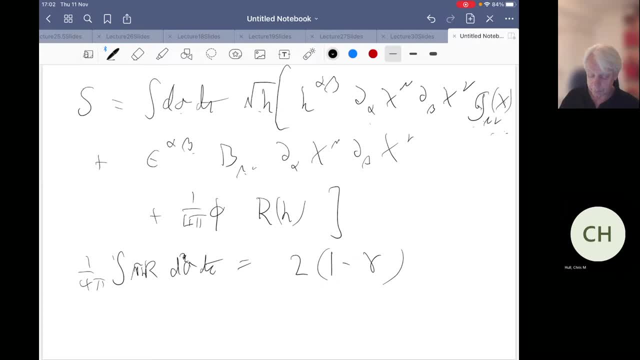 two into one minus the genus. so here i'm thinking of going to having gone to a euclidean signature on the world sheet. so h is a positive definite metric, um, so tau is the euclidean time and the integral of the curvature. um turns out, rather remarkably, to be a topological quantity. 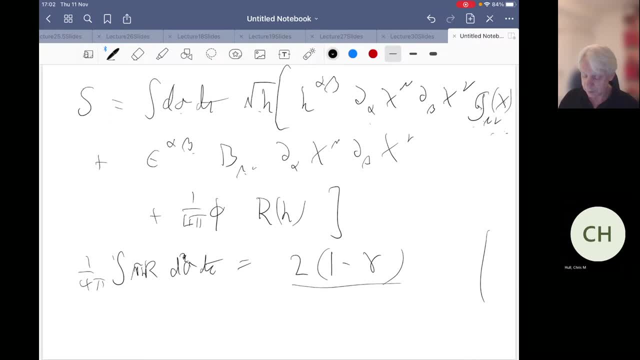 and it gives precisely um 1 minus the genus times 2.. so this means that if we look at um the b to the minus the x, the action, then this has got a term, and if we think of the scalar field, dilaton as. 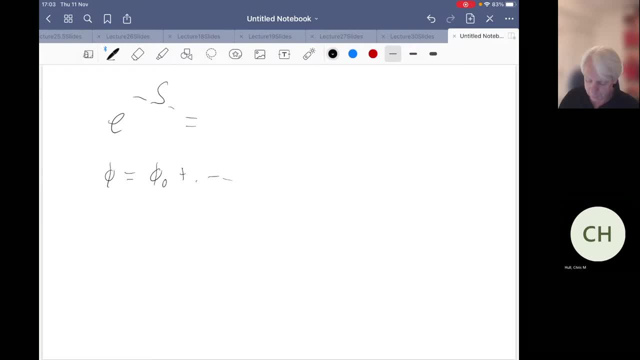 being a constant plus some other pieces. if we look at the constant piece, we get e to the minus integral pi, zero, r plus other terms with 1 over 4 pi, and this is equal to e to the minus 2 pi, zero to the 1 minus gamma. 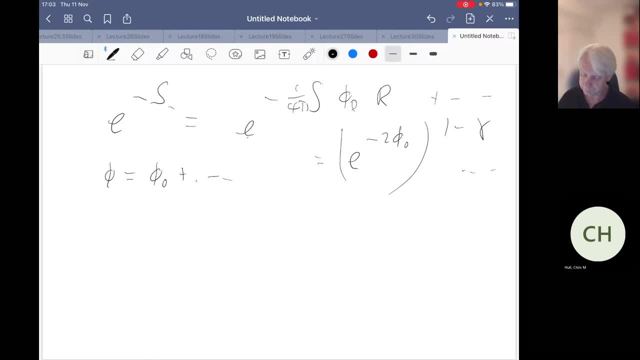 So this term is that times the terms which come from the other fields, from the non-constant parts of phi and the other fields in the theory. But this action, if we look at the phi zero dependence, it comes with a factor like this. So we see that if we look at this. so this is 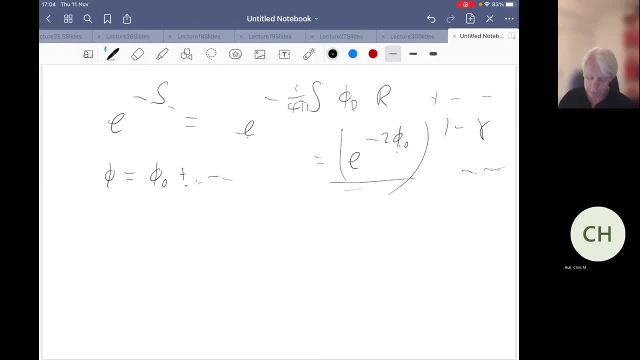 precisely the same way in which the g squared appeared. So in fact we find that at genus minus gamma we get a power of g squared to the gamma minus 1, and e to the minus 2 phi zero. so e to the plus 2, that to the gamma minus 1.. So now we see that g and phi zero always. 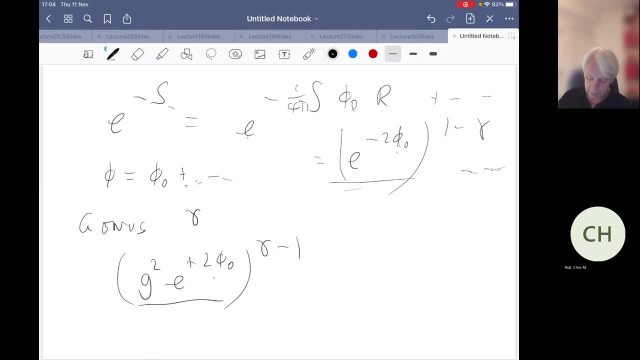 enter in this combination And so there's a symmetry under which you take g goes to lambda g and phi zero goes to phi zero minus c, minus lambda. So you scale g and shift phi zero. So that means that g, which is the power of g, can be absorbed into phi zero And we don't need to talk separately. 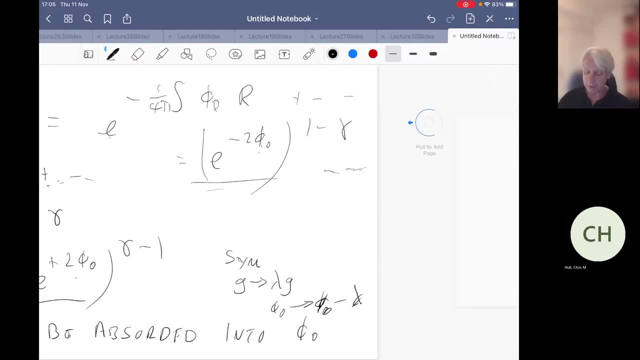 about the coupling constant, Or rather you can think of the strength of the coupling constant, which there is some calculation for cap момент, in a least disagreement that we can think of, at g, being given by the expectation value of e to the phi. And more generally, we can think: 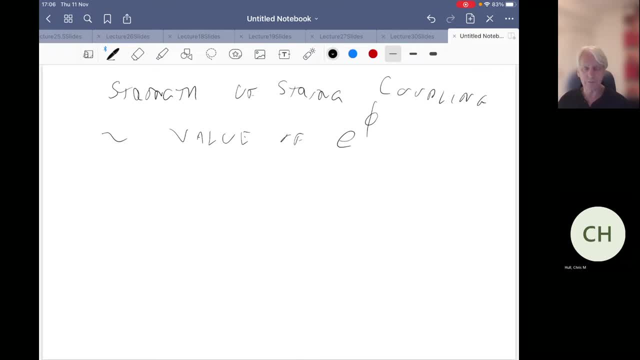 if we have a varying background where the dilaton is weak in some areas and strong in others, we can say that there's some regions of the background in which the string is weakly coupled and others where it's strongly coupled, And this is a general feature in string theory. 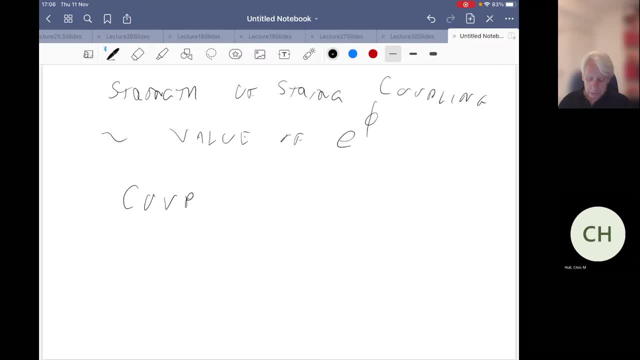 that the coupling constants- and I'll say more about what these are in a moment- all come as vacuum expectation values of scalars, And so that gives us a very nice way of so the the some ways there's. there aren't independent coupling constants, there's rather just scalar. 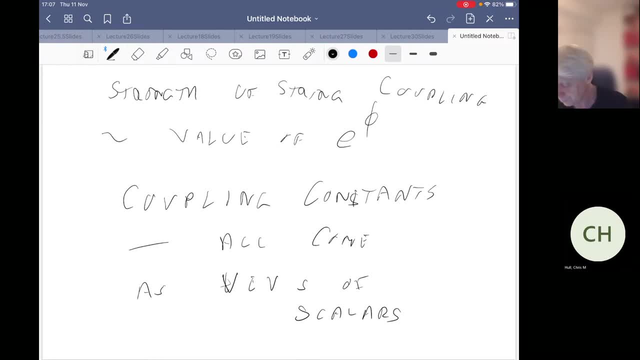 fields and expectation values determine strengths of coupling. so now we come to the question about that we started with. if we think about strings, before 1994 string theory theory was defined as a perturbation theory and it gave a prescription for calculating and scattering of string states. 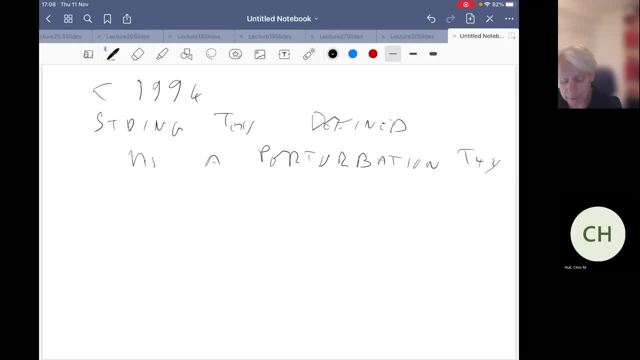 perturbatively in the coupling constant, and it gave a very nice picture. and it turns out there were five different, distinct perturbation theories, all of which seem to give consistent theories, and so i want to return now to what happens if, as g, gets larger, so that the perturbation theory may or may not be. 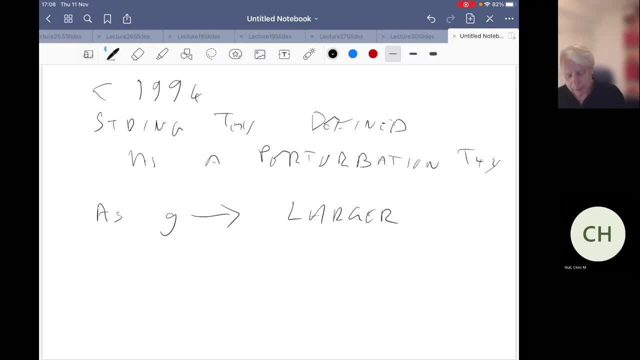 not, may or not be valid. so let's first let's think in some generality about both field theories and string theories. first of all, in general, in field theories the coupling constants will get renormalized, so they will get dependent on energy or temp or temperature, and 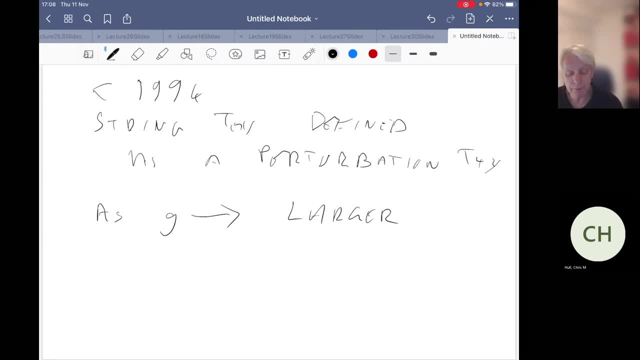 so as a result, even if you started off with one, one small value of the coupling constant, as you change the energy or change the temperature, then that value might grow, and so you need to confront what happened in other values. so, for example, in qcd, um, at high energies or high temperatures it's weakly coupled, but as one. 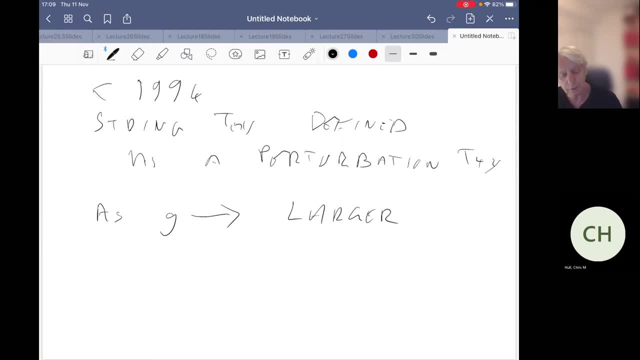 reduces the temperature, it becomes more and more strongly coupled, and so one needs, and so the picture one has of it changes, one's forced to, uh, to confront the issues of strong coupling. um, however, some theories, um, for some theories, the coupling constants are not renormalized. 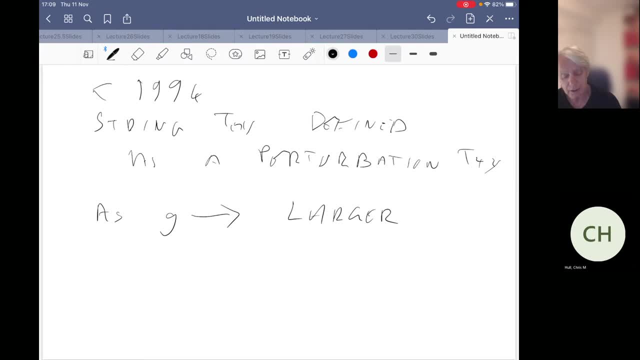 if, in particular if supersymmetric theories which are finite- for example n equals four super yang mills- the coupling constant does not get renormalized. it's a, so it becomes a parameter which just um parameterizes the theory, and we can think about the theory for different values. 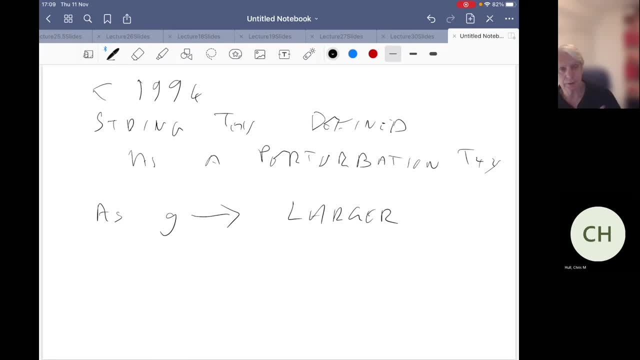 of the parameters, and the same is true in string theory, but there's but, as we've just seen, the escape. the coupling constants arise as expectation values of fields and because we can, we want to consider arbitrary field configurations. we're forced to think about what happens, um if, um, if the configuration where the coupling constants are large, 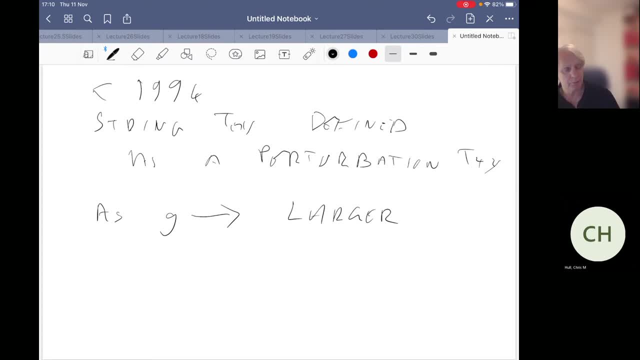 so a big role is in in the presentation was played by the um, free fields, uh, the free field limit, where we take the coupling constant to zero and we get the fundamental degrees of freedom, at least for the perturbative theory. but as one um increases the coupling constant, there's a question about whether the fundamental 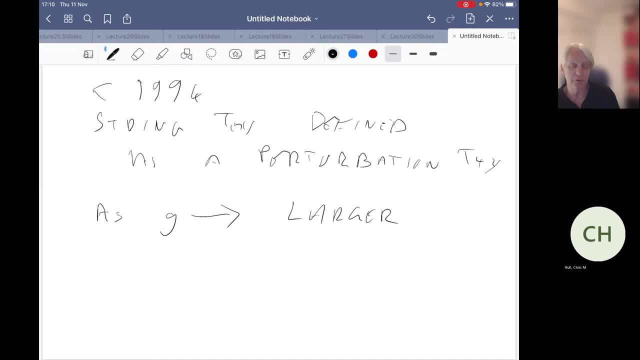 degrees of freedom remain the same and for many theories what happens is that some of the degrees of freedom, some of the particles, may become unstable as you turn up the strength of the coupling and in particular in string theory, many of the massive string states turn out to be unstable. 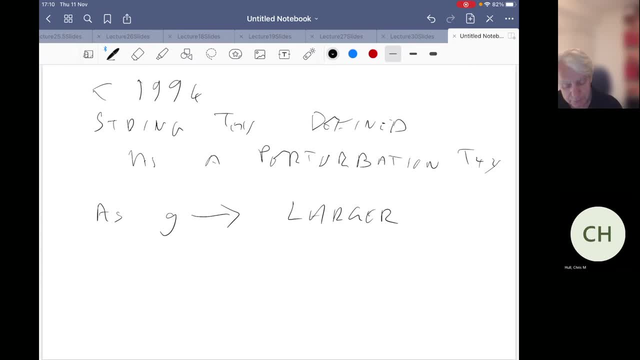 as one turns up the coupling, and if uh and so states which are in the perturbative string spectrum for small coupling will not be there for large coupling, and so there's a question about what the right set of fundamental degrees of freedom might be in general, in theories. then as you turn up the coupling, there may also be. 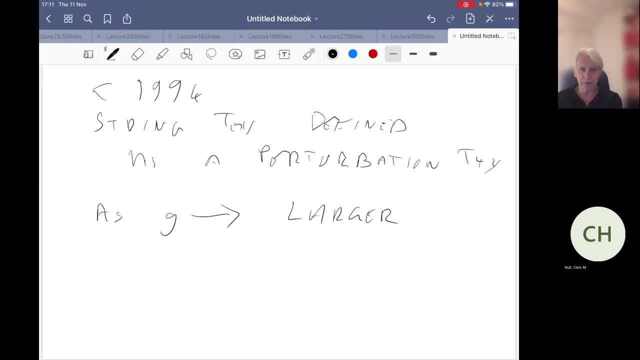 phase transitions, so that you might get a completely different physics and completely different set of fundamental degrees of freedom. another related question is whether you can, whether the theory is actually defined for all values of g, of the coupling constant, or whether there's some maximum value of the coupling constant and what happens as one turns that up. 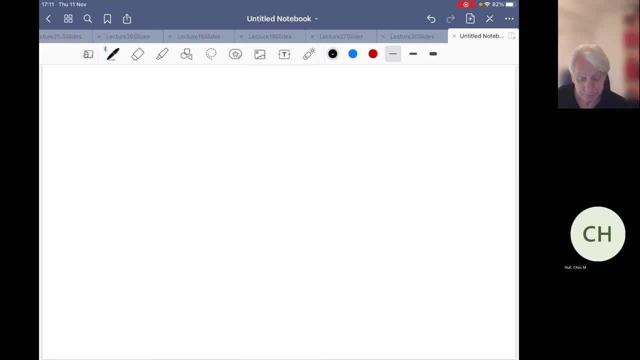 so um, if um, if the theory is defined for all values of the coupling constant um, we can then consider um. so suppose theory define for all values of the coupling constant. as um g becomes very large, one over g is small, obviously, and you can ask um whether, whether we can think, can we?